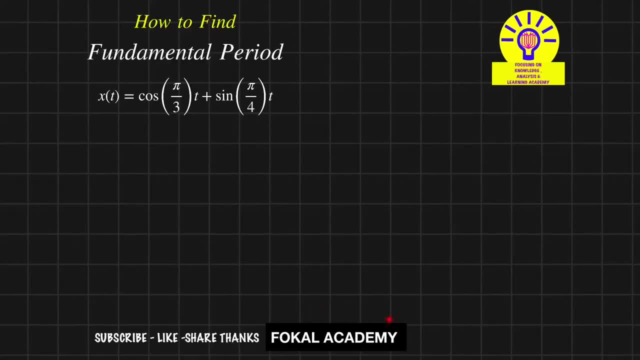 Hi everyone, welcome to focal academy. See in this problem here how to find fundamental period for signal x of t. Here again, x of t is a combination of two signals, that is, cosine signal and sine signal. So let consider that this is x1 of t signal and this is x2 of t signal. So first of all find the individual fundamental period for x1 of t and x2 of t, So then we can easily find the fundamental period. 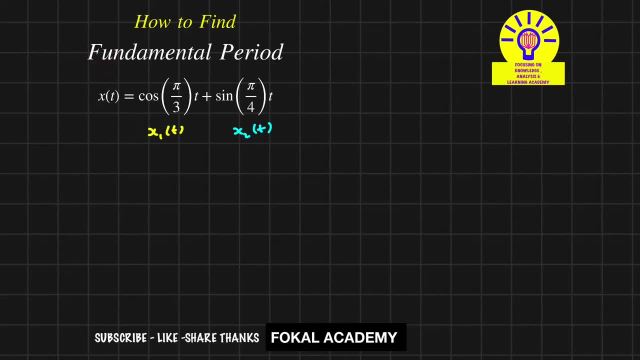 For given signal. So let consider t1 be the fundamental period for x1 of t, that is equal to 2 pi by omega 1.. So here this is the omega 1 value. Now substitute here and it becomes 2 pi by pi by 3.. Nothing but t1 equal to 6.. Similarly, t2 equal to 2 pi by omega 2.. And this is the omega 2 value. 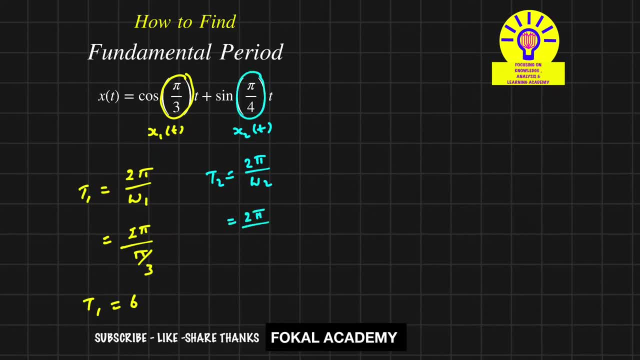 Now substitute here and then becomes 2 pi by pi by 4.. By simplifying this we will get 8.. And this is the t2 value. So before finding the fundamental period, check the given signal is period or not period. So that is t1 by t2 equal to here: t1 we got 6 and t2 we got 8.. By simplifying this we will get 3 by 4.. So it is the rational number. So then we can say that the given signal is 2 pi by pi by 4.. And this is the t2 value. 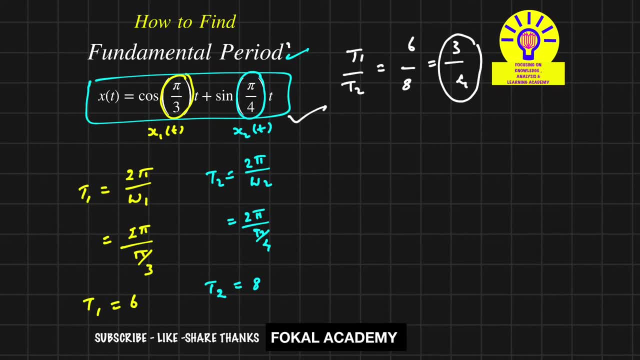 signal is a periodic. that means we can find the fundamental period now cross mod plate and it becomes four t one and that is equal to three t two. it is nothing but fundamental period for x of t signal. now take any equation now substitute in that t one or t two, then 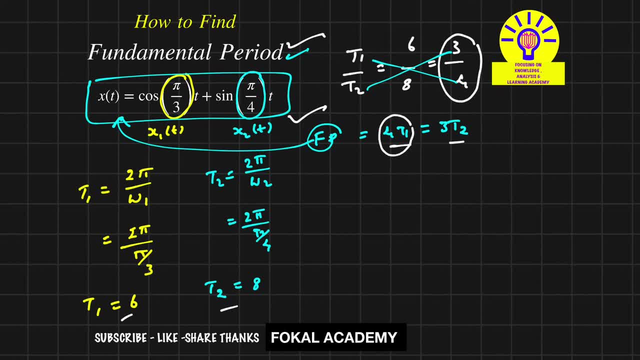 we get the fundamental period now i am going to take four t one, that is, four, into t one- we got six- nothing but twenty four. or take three t two- nothing but three into t two- we got eight- nothing but twenty four. so this is the fundamental period for signal x of. 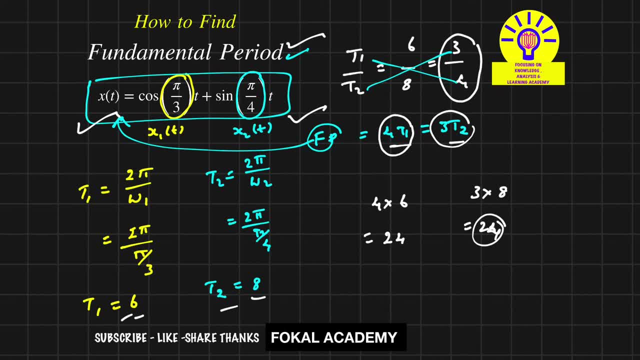 t and this is the process of simplification and thanks for watching. please subscribe like, share, thanks.